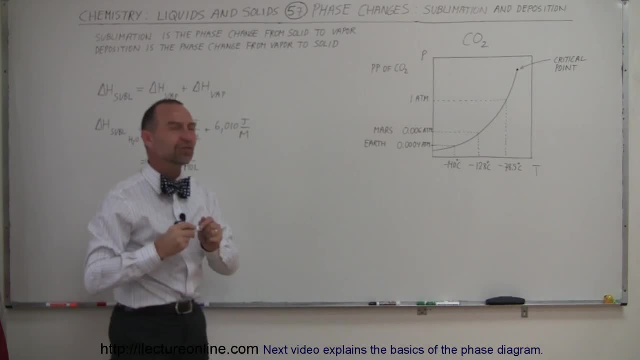 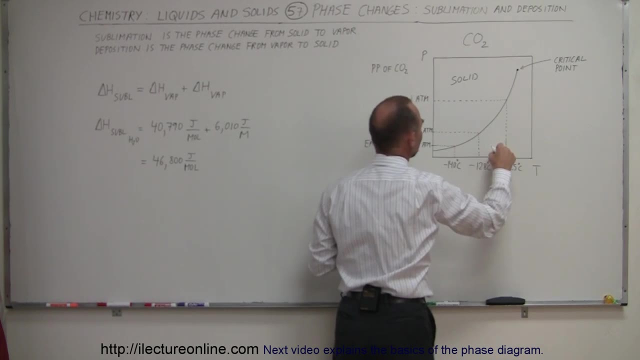 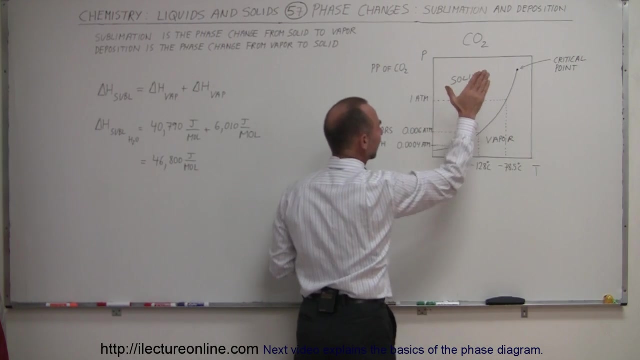 dioxide. And here I have a phase diagram for carbon dioxide, at least a partial phase diagram, which shows the relationship between what we call solid carbon dioxide and vapor carbon dioxide. So notice our phase diagram here, where we have this relationship between solid carbon dioxide and vapor carbon. 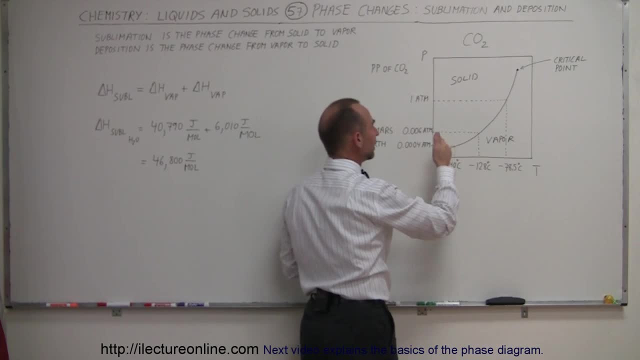 dioxide, And also notice that the way the pressure at which this happens does depend upon the temperature, or vice versa, The temperature at which it happens does depend upon the pressure. That may be a better relationship. So notice that at one atmosphere- so that would be the atmospheric pressure of the Earth- vapor carbon dioxide will turn into. 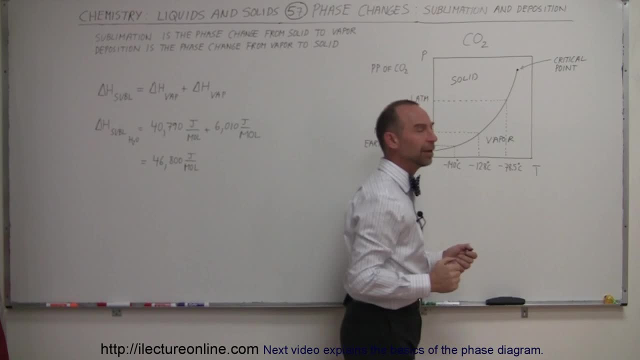 solid carbon dioxide if the temperature drops below 78.5 degrees. But that's a little bit misleading. The reason why that's a little bit misleading is it doesn't depend upon the total atmospheric pressure. It does depend on the partial pressure of carbon dioxide in the atmosphere And 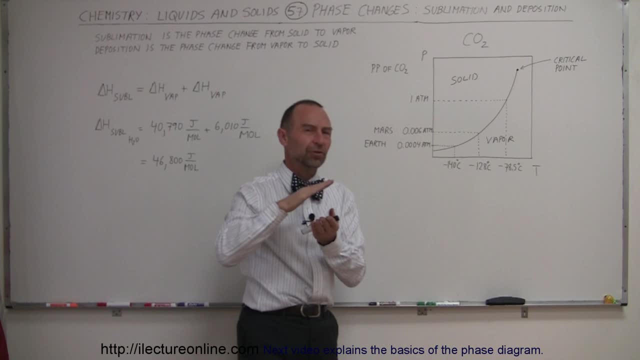 for the Earth. there's not a lot of carbon dioxide in the atmosphere, so the partial pressure of carbon dioxide is very, very low. So, assuming that we put carbon in a container- or carbon carbon dioxide, I should say- in a container in a vapor form, and let's say that the container is 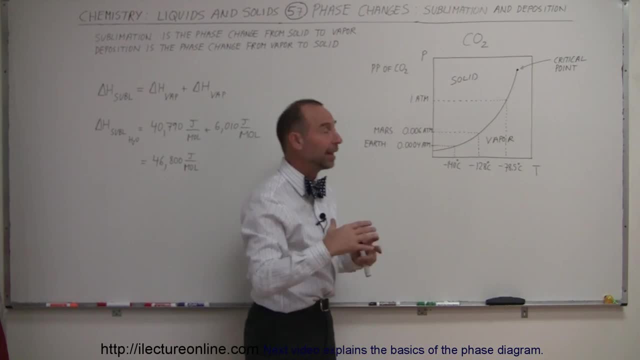 completely filled with carbon dioxide and now we apply pressure to that, then we can assume, of course, that we start out at one atmospheric pressure and then, if we cool it down down to 78.5 degrees, that carbon dioxide will turn into a solid at one atmosphere, But on the Earth. 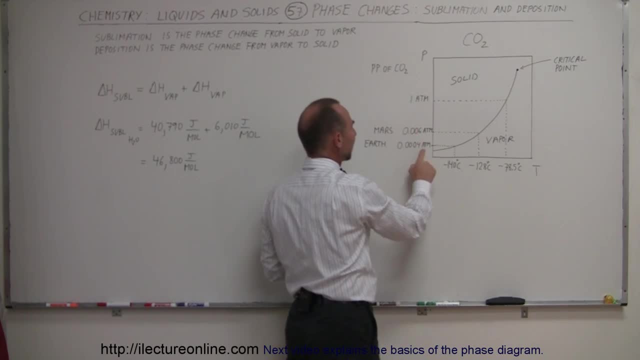 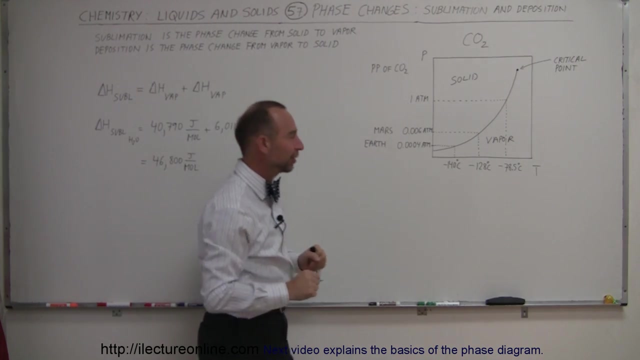 the partial pressure of carbon dioxide is only 0.0004 atmospheres, So it would have to get to 140 degrees below zero centigrade for vapor carbon dioxide- the carbon dioxide in the atmosphere, actually precipitate out like snow and fall down to the earth. never does it get that cold on the 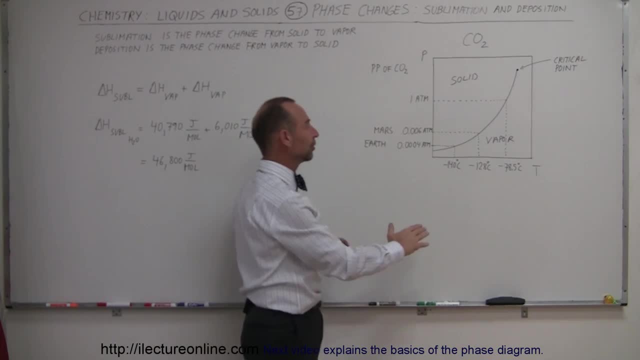 earth anywhere, not even in the antarctic, not even in the closest place of the world. so we'll never on the earth see carbon dioxide precipitate out as snow and fall down to the ground. but it does happen on mars. on mars, the total atmospheric pressure is much lower than the earth it's about. 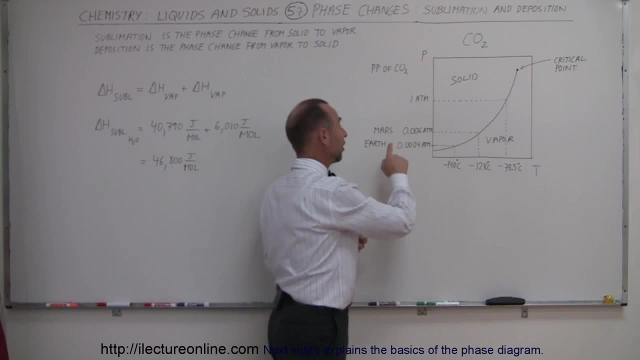 0.6 percent of the atmospheric pressure on the earth, but almost all of that is carbon dioxide. so you can say that approximately the partial pressure of carbon dioxide in the martian atmosphere is about 0.006 atmospheres, which means that at the temperature of 128 degrees below zero, 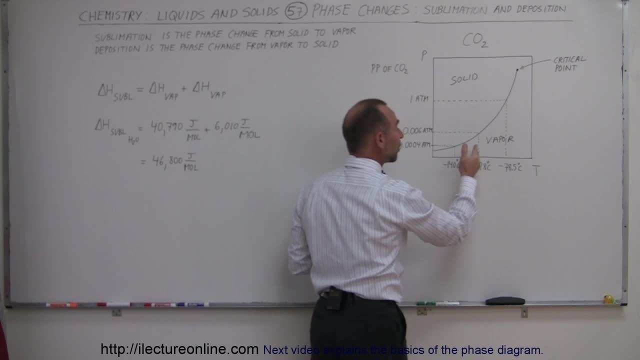 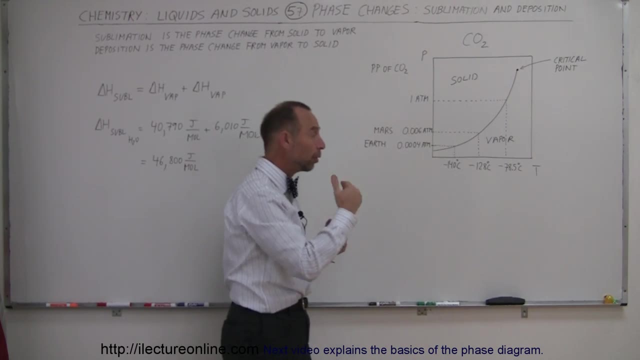 centigrade degrees, the carbon dioxide vapor will indeed turn into solid carbon dioxide. so on places on mars where, in the winter time near the poles, it gets so cold that the temperature drops below this temperature minus 128 degrees centigrade, and carbon dioxide will actually precipitate out of the atmosphere and fall down to the ground like snow, and so the 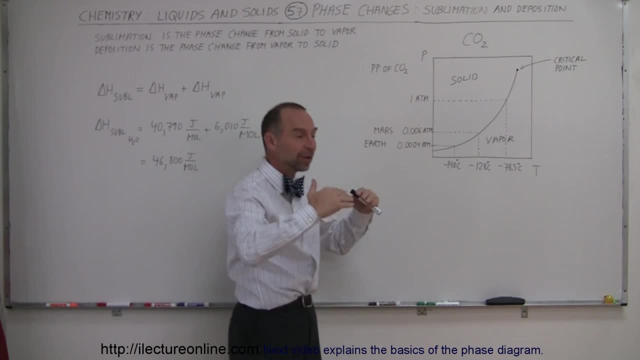 polar ice gaps will build up over the winter time, but instead of building up with water ice, they build up with carbon dioxide ice. so they get much bigger in the winter time because of the precipitation of carbon dioxide out of the atmosphere and then in the summer time in the 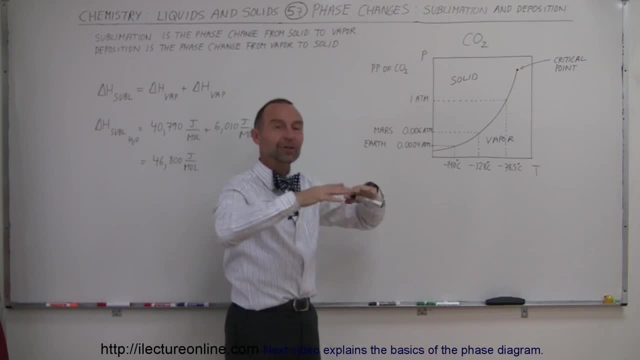 spring and summer time it sublimates again there, goes directly from the solid form carbon dioxide back to the vapor phase of carbon dioxide and disappear again into the atmosphere. and this happens every winter and every summer at both poles on mars. so again, it does depend upon the 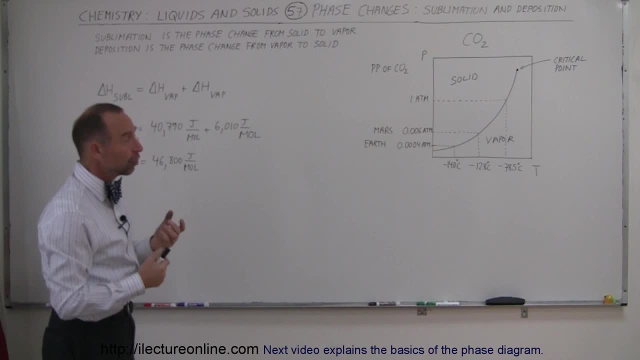 temperature and the pressure, so sublimation occurs. there's a number of substances that sublimate not a lot. there's a number of substances that then deposition again when the temperature gets cold enough, and again it all depends on the partial pressure of that vapor in the atmosphere. 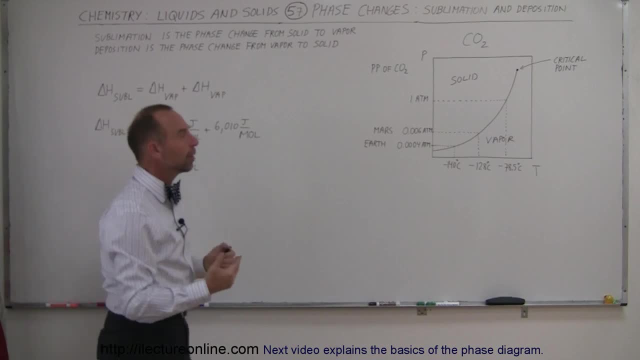 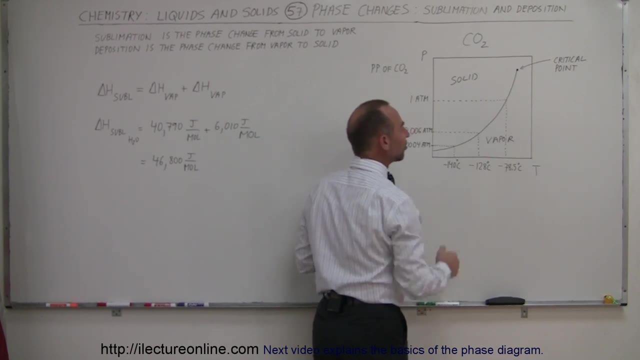 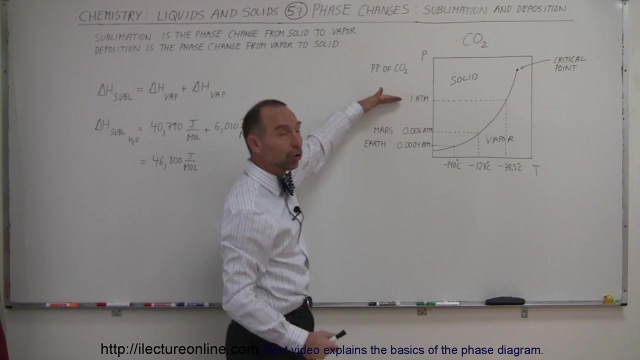 not the total pressure, because that's quite often misunderstood. we always think about the- the temperature at which uh carbon dioxide sublimates on the earth- as being minus 78.5 degrees centigrade, because we associate that with a pressure of one atmosphere. but it's incorrect to assume that it depends on the total atmospheric. 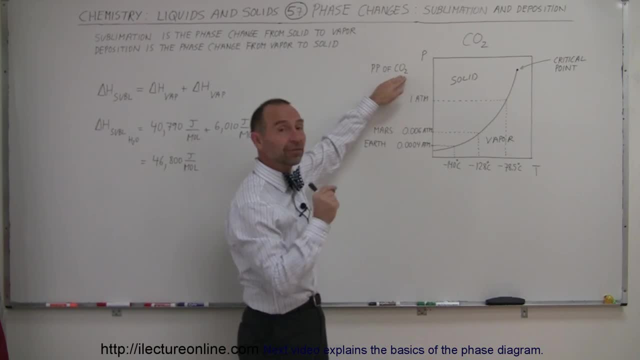 pressure. it only depends on the partial pressure of the carbon dioxide vapor in the atmosphere, but that controls the amount of sublimation. so on the earth the temperature which it happens is minus 140 degrees centigrade, not minus 78.5. and the way they do turn carbon dioxide into solid carbon dioxide is typically by cooling it. 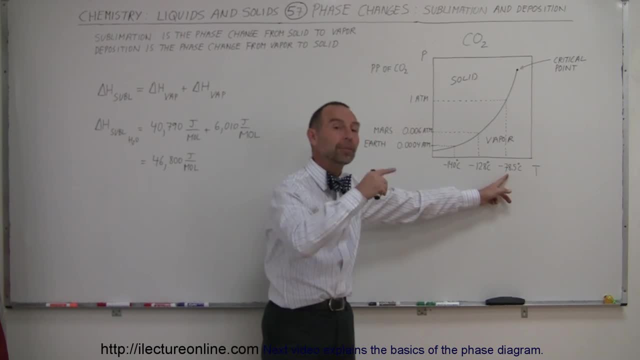 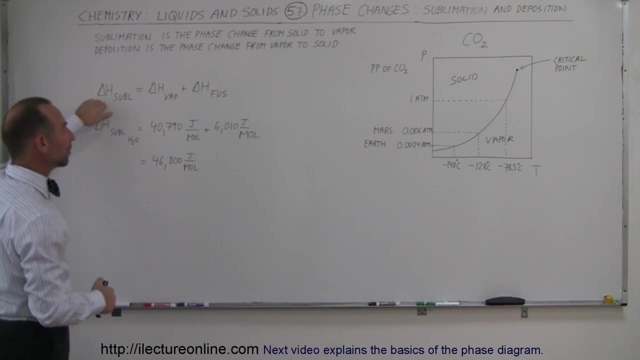 to a very, very low temperature, minus this, assuming that the partial pressure is entirely the atmospheric pressure in that particular container. here we have the enthalpy of sublimation, which is the amount of energy required, because it does require energy to turn solid carbon dioxide into.